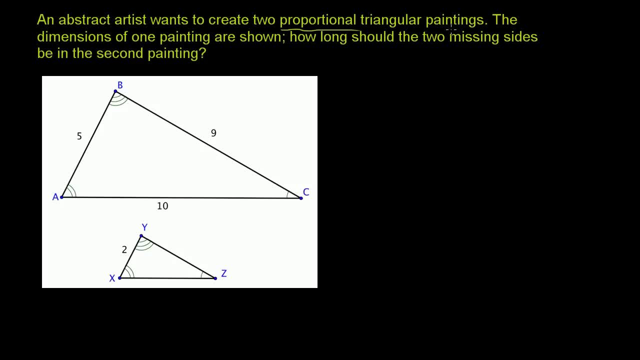 An abstract artist wants to create two proportional triangular paintings. The dimensions of one painting are shown and that's this top one right over here. How long should the two missing sides be in the second painting? So there are two proportional triangular paintings, or one way to think about it. 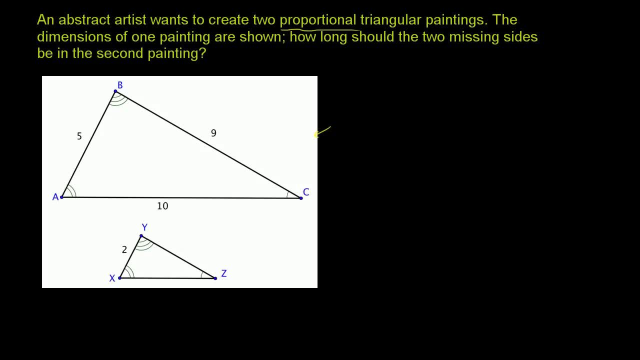 is going to be two triangles that are similar And actually we know, based on how these triangles are marked up, that they are similar triangles. You have this angle with these two arcs right over here. It has the same measure as that angle right over there. 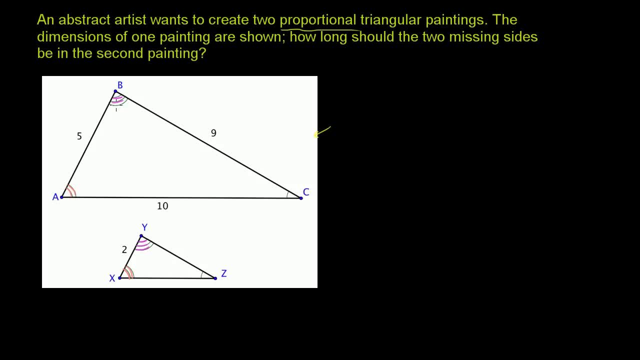 This angle with the three arcs has the same measure as this angle right over there And that this angle- let me do it in a new color with the one arc- has the same measure as this angle right over there, If the corresponding angles have the same measure. 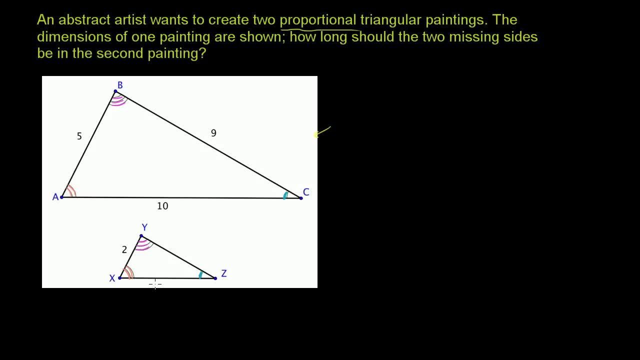 if the corresponding angles are congruent, then we know that these are similar triangles. The other thing that tells you about similar triangles, or if you know that two triangles are similar, that means that the ratio between corresponding sides is going to be the same. 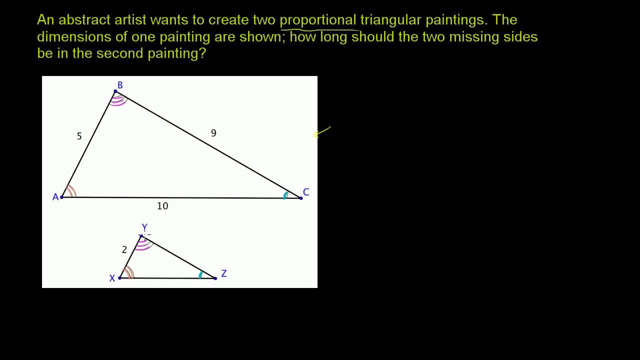 So let's look at the corresponding sides and then let's try to figure out that same ratio, or use that same ratio so we can figure out the missing sides right over here. So the first thing, if you look at the side that's opposite. 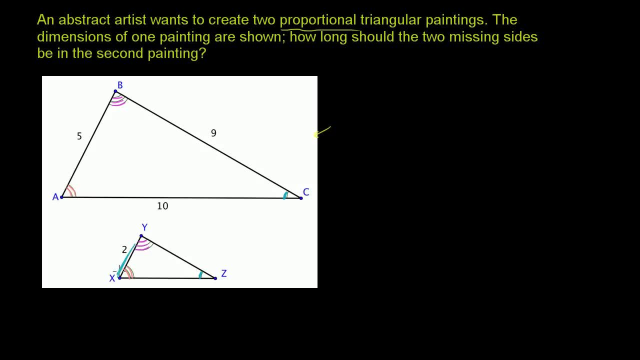 this blue angle, this one arc angle, side xy over here. that's going to correspond to the side that's opposite this blue angle over here. so side ab, These are corresponding sides. You could also view it as a side between the orange. 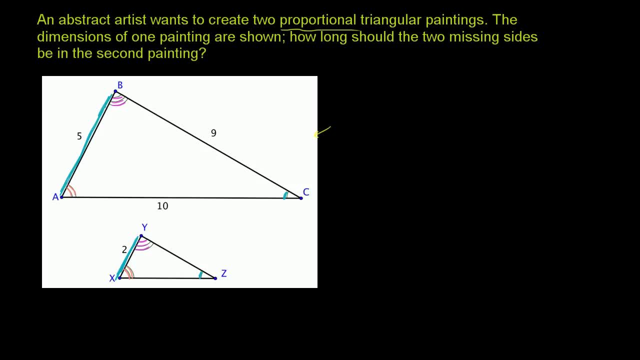 and the magenta, the side between the orange and the magenta. Likewise, this side right over here. that's opposite the orange angle. it's opposite the orange. the double arc angle is going to correspond to this side. that's opposite the orange double arc angle. 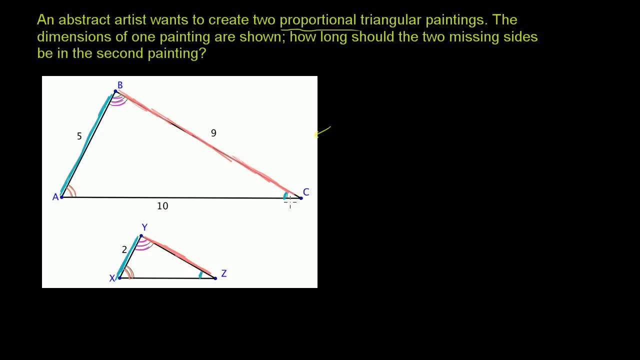 Or you could view it as a side that's between the magenta and the blue angle. And then, finally, we have this side which is opposite the magenta angle. It's opposite the magenta angle, It's between the blue and the orange angles. 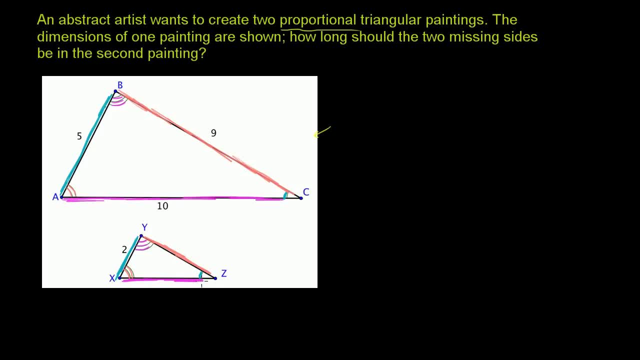 It's going to correspond to this side which is opposite the magenta angle, and between the blue and orange angles. So what this tells us is that the ratio we know, since they are similar, the ratio between corresponding sides- is going to be the same. 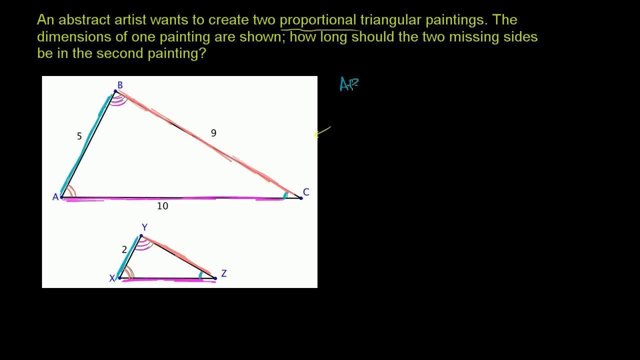 So the ratio between these two sides, ab to xy, the ratio between the length of side ab and length of side xy, is going to be equal to the ratio between the length of side bc and the length of side yz, Which is going to be equal to the ratio of ac to xz. 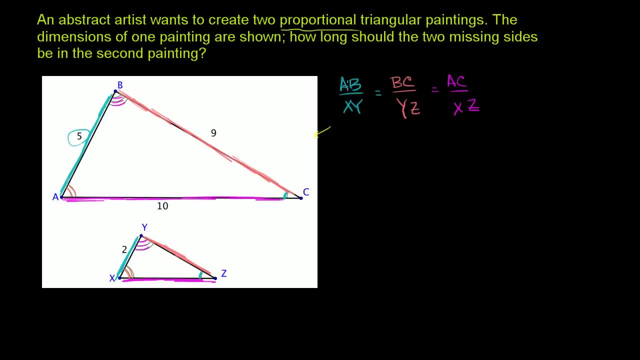 And they tell us what some of these lengths are. They tell us ab is equal to 5.. They tell us that xy is equal to 2.. They tell us that bc is equal to 9.. And yz is one of the things we're. 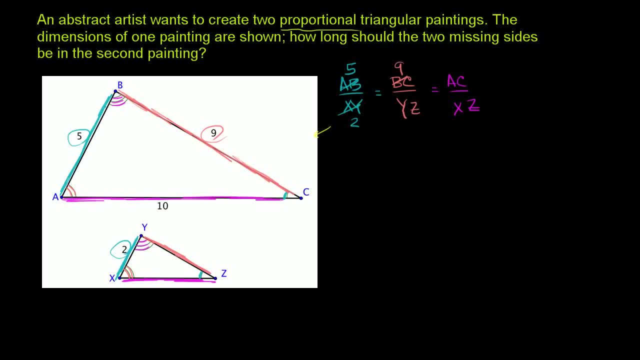 going to have to solve for, But they also tell us that ac is equal to 10.. I want to use the magenta. ac is equal to 10. And we also have to solve for xz, So we can actually get this triple equality. 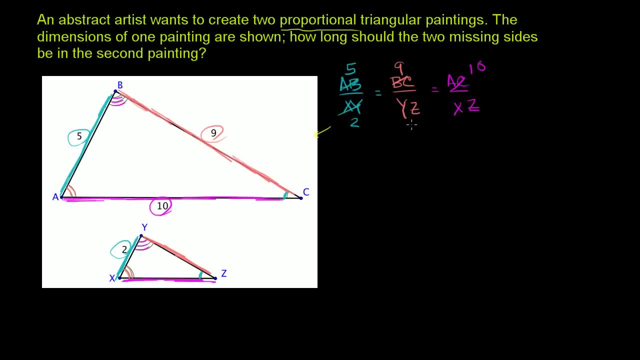 We can actually create two separate equations, each of which have one unknown, And then we can solve for that unknown. So the first is you have 5 halves is equal to 9 over yz. And to solve for yz there's a bunch of ways. 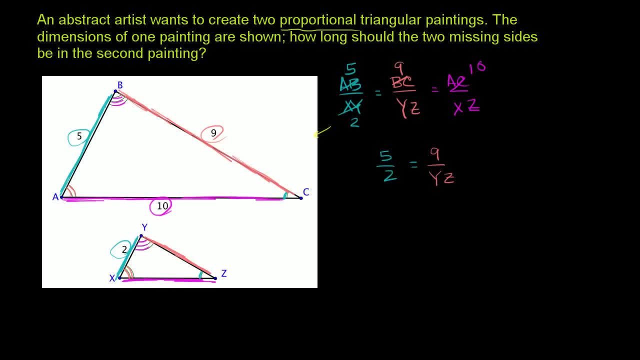 that you could do. You could do it, but you could just. let's see, we can multiply yz times both sides- And actually I won't, well, and then we can multiply both sides by 2 fifths, But let's just do one step at a time. 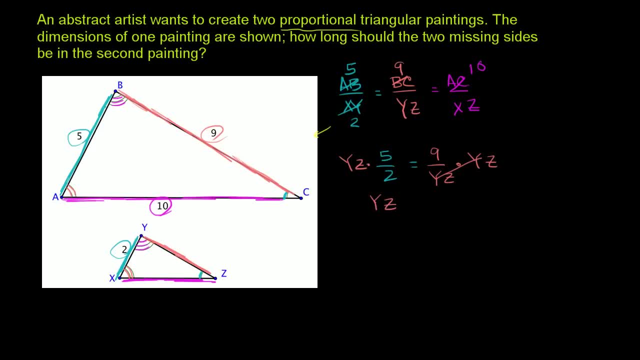 So then you get: yz times 5 halves is equal to 9.. And then you can multiply Both sides times the reciprocal of 5 halves. So you multiply both sides times 2 fifths. And we're doing that so that we can isolate the yz. 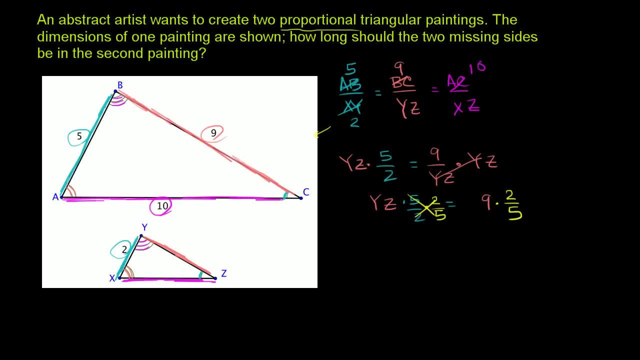 And then this right over here: these cancel out. On the left-hand side we're left with just yz, And on the right-hand side we are left with 9 times 2 is 18 over 5. And we can turn that. 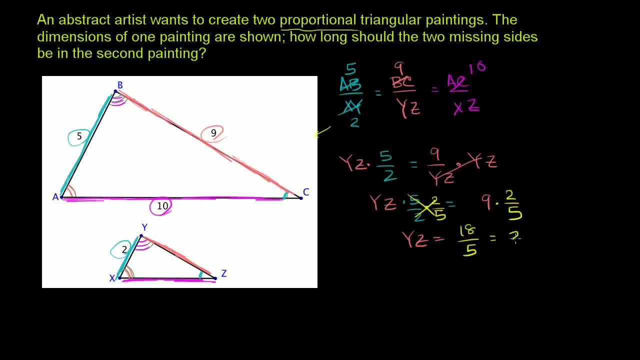 This is the same thing. if we write it as a mixed number, 5 goes into 18 three times, With a remainder of 3.. So it's 3 and 3 fifths, which is the same thing as 3.6.. 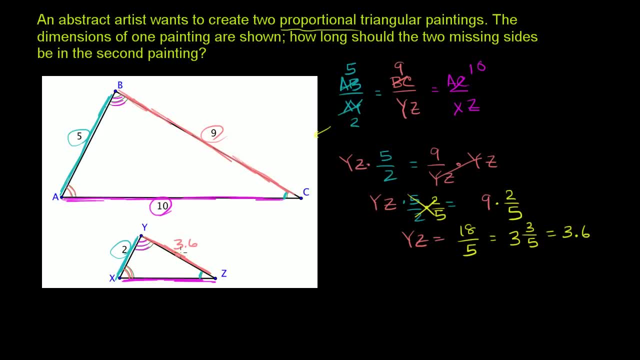 So yz over here is going to be 3.6.. So we've done one of the sides. Now we have to figure out what xz is, And so here we know that 5 halves is going to be equal to 10 over xz. 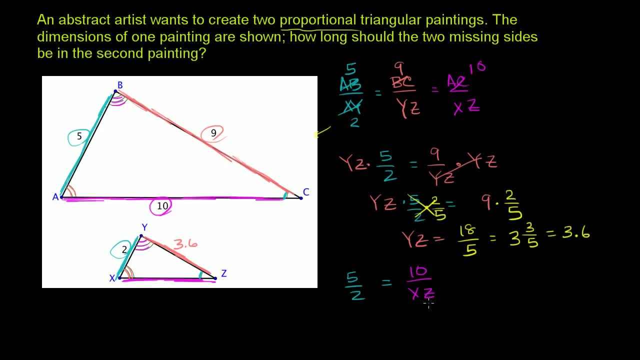 And once again, we can multiply. There's multiple ways you could do it. You could flip both sides of this equation, So you could say so, I'll do it in a slightly different way than we did it that way, just so. there's multiple ways. 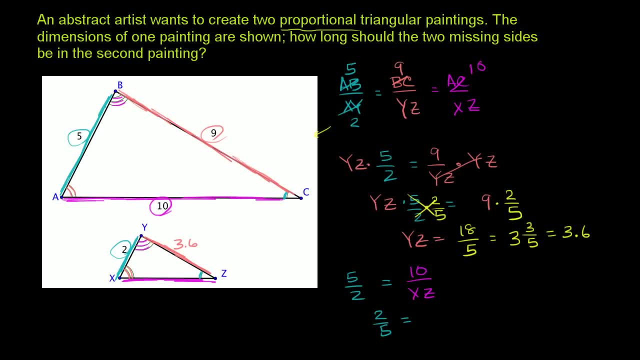 to solve this You could say: 2 over 5 is equal to xz over 10.. So I'm just taking the reciprocal of both sides And then multiply both sides of this equation by 10.. Multiply both sides by 10.. 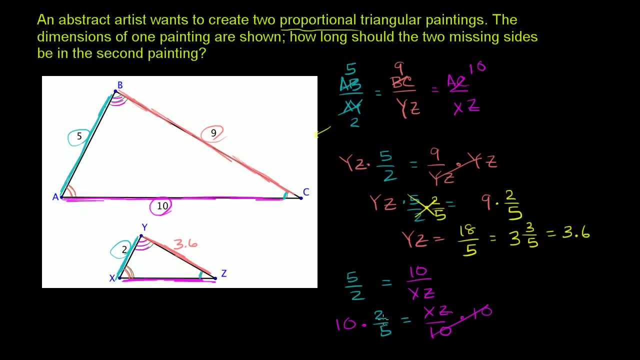 So you're left with. xz is equal to 10 times 2, is 20 divided by 5.. So this is going to be 4.. So xz ends up being 4.. So xz ends up being 4.. So xz ends up being 4.. 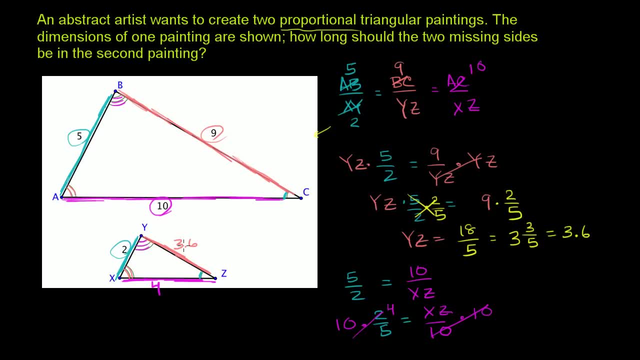 That is 4.. And we're done. The smaller painting has dimensions 2,, 3.6, and 4.. 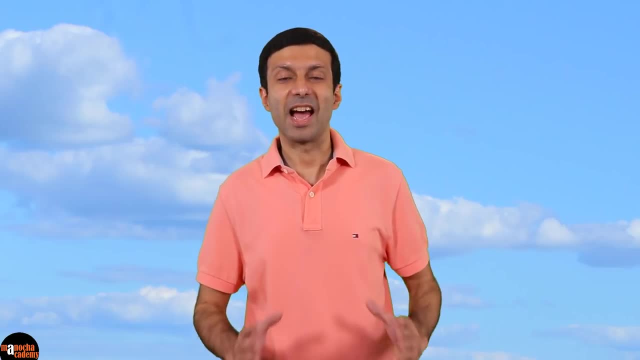 Hi friends. let's say you're standing near a tall building and you want to measure its height. Let's say you're in front of Burj Khalifa, which is the tallest building in the world, So how do you measure its height? Or let's say you're standing on a bridge across a river. 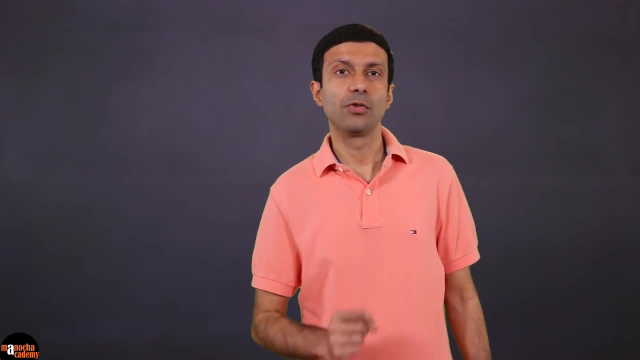 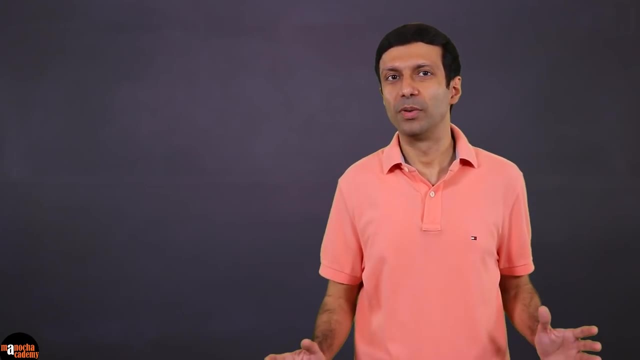 How do you measure the width of the river? To measure the height of a tall building, we'll have to go to the top and drop a long rope and measure the length of the rope, So it's not convenient, right. Measuring the width of the river is even harder. 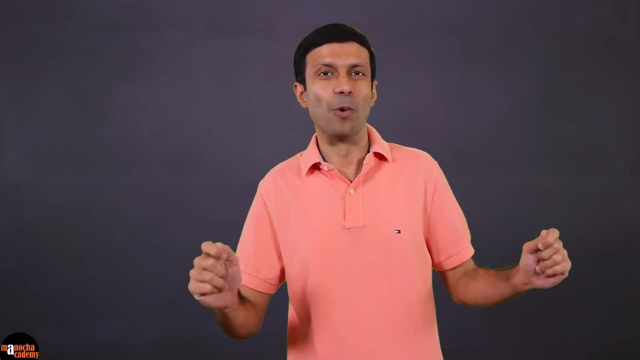 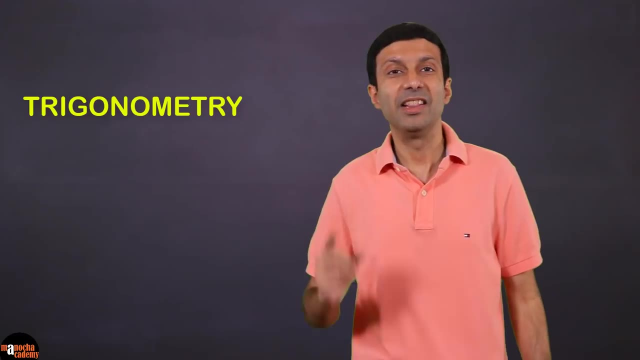 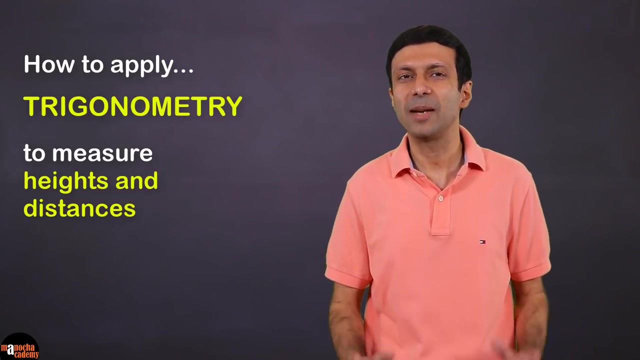 because you have to stand on opposite banks with a long rope, So it's not practical. But if you know trigonometry then it's really easy. In this video we'll learn how to apply trigonometry to measure heights and distances. I'm going to make the concepts really easy for you.